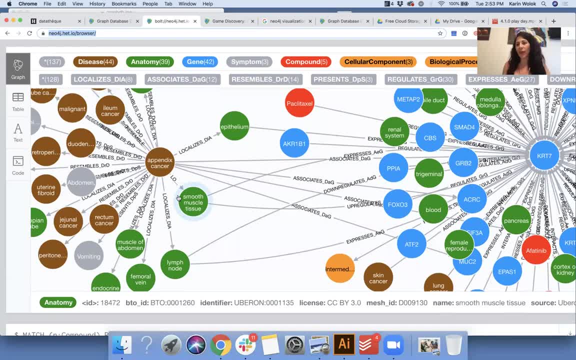 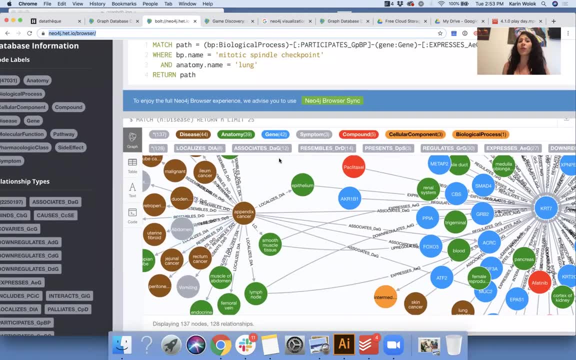 my screen. So this is an example of like the Neo4j browser right here. So one thing that I think is really important to note, very important to understand, is that Neo4j is a database- Okay, That is. it's not a visualization that sits on another database. 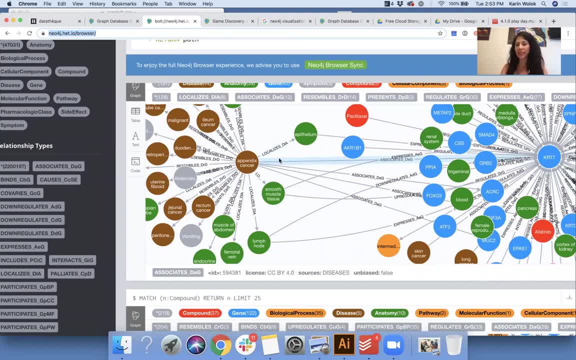 It is an asset compliant transactional database, So that's something that's very important. Technically it's in the NoSQL category, but it's very, very different from most normalized relational databases in the sense that most relational databases store data in the shape. 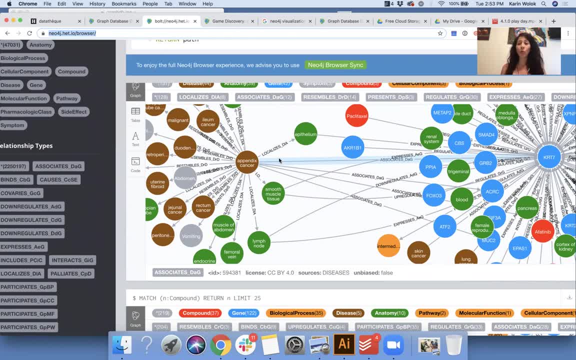 of tables and joins. Neo stores the data in the shape of a graph, And when I say graph I do not mean a chart, I mean a graph theory, graph like a network. So in the data model inside of Neo4j is like: 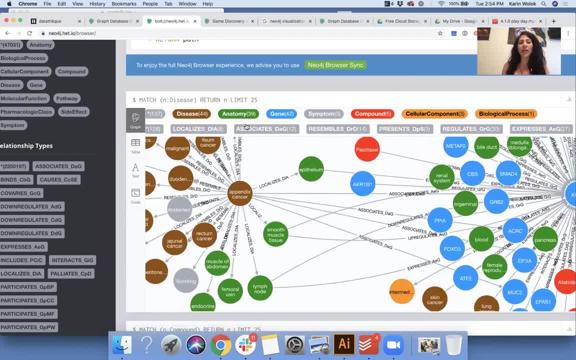 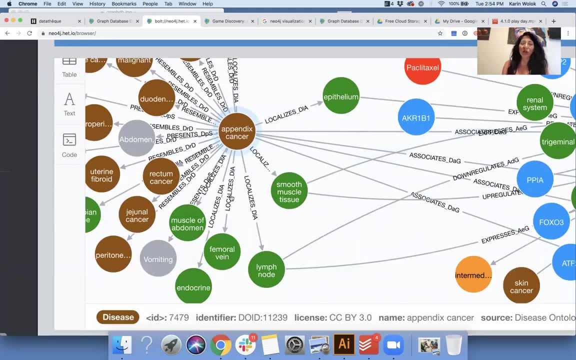 you have your nodes here. Your nodes are your nouns, That's person, place, thing, location, right. These are your nodes, your nodes here And then. and these nodes could also have properties which they could be like labeled right here. So those are your properties, And then you can have. 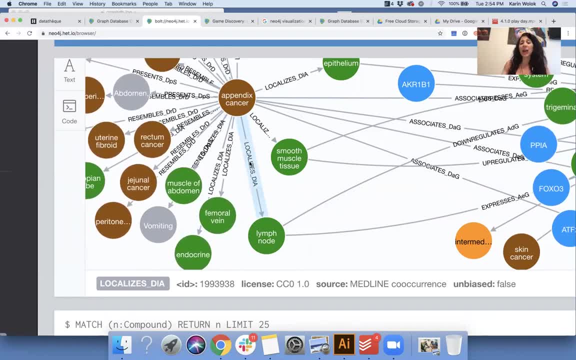 relationships between those nodes and those relationships are- and in Neo4j relationships are- actually first-class citizens, meaning that they are just as important as the nodes themselves, like how are things connected, right? So just like you could have different types of nodes, you can also have different types of relationships. You can put. 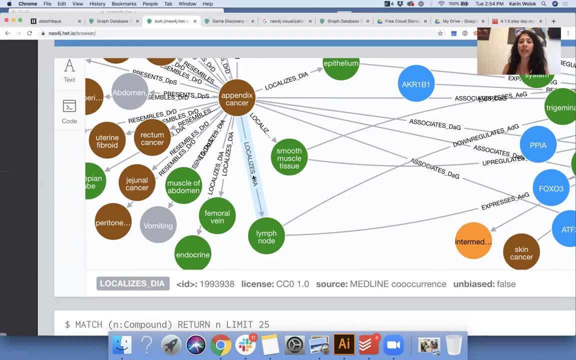 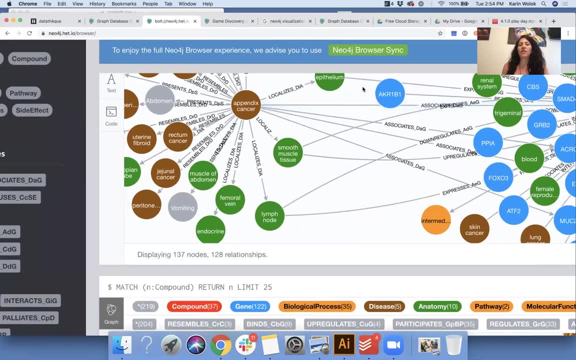 properties in those relationships. You can put values so they could be weighted, You can have geospatial information, You can have date and time. So basically, whenever you have data that's complexly connected and you want to understand how these things are connected to each other, 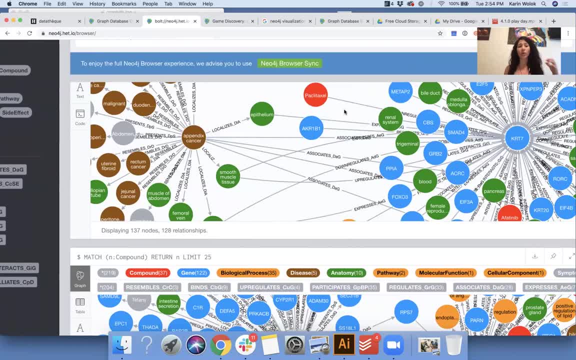 or maybe you want to find a shortest path- right, Like shortest path from here to here. or maybe you're looking for patterns in your data, Or maybe you're looking for something that's like a combination of patterns, right, It might be like 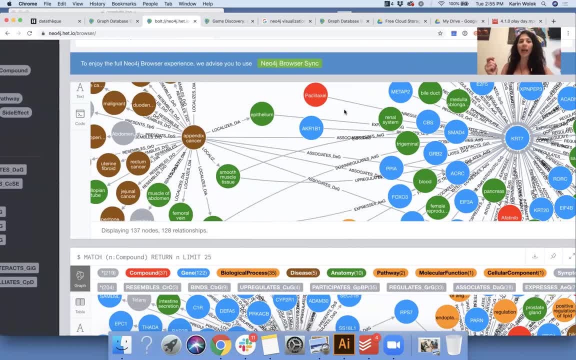 if you're doing fraud detection, it might not be one transaction that sets off a flag, but it's a transaction with these other patterns that in behavior that might be kind of you know, raising the flag, Or if you're doing any kind of graph algorithm type of analysis. 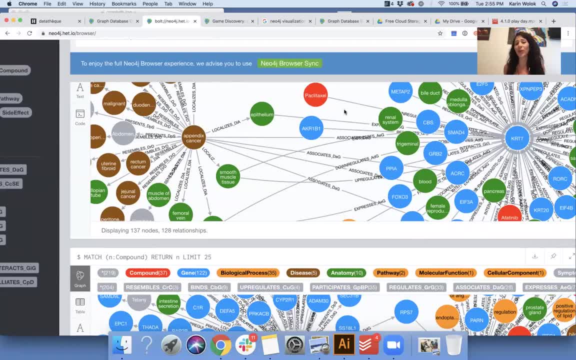 whether you're like community detection or between the centrality and page rank things like that, like network related style queries, like is the shape of your data network or is it a table? So that's kind of like the big differences. So there's a few things that 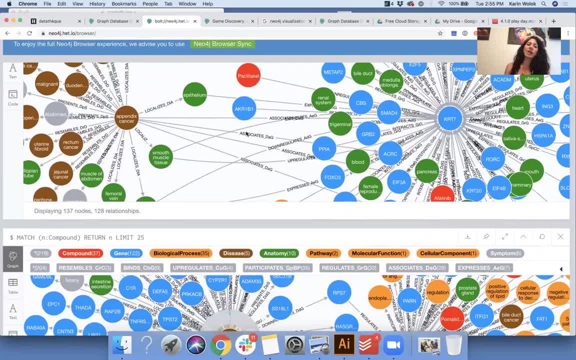 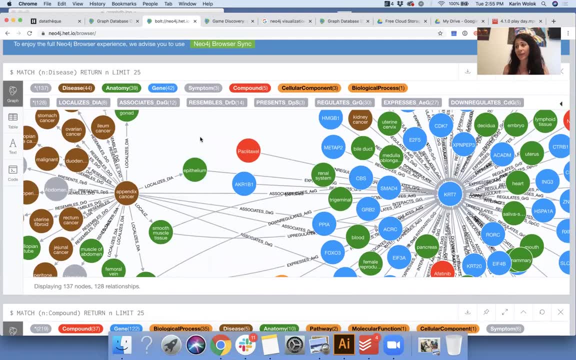 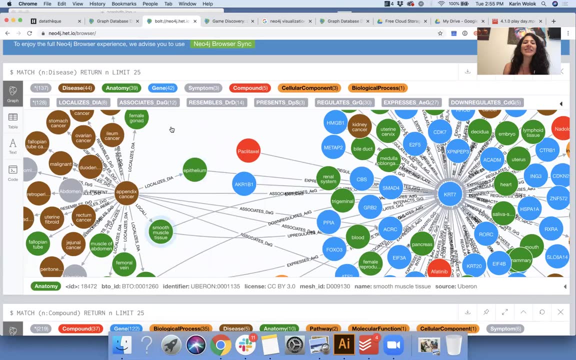 I think that are really important to note about understanding Neo4j and what makes it different. So, for one thing, Neo4j is a native graph database, And what that means is the underlying architecture of how the data is actually stored is not built on top of tables. Everything is built. 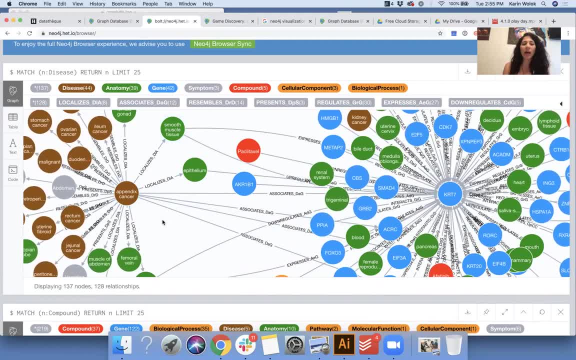 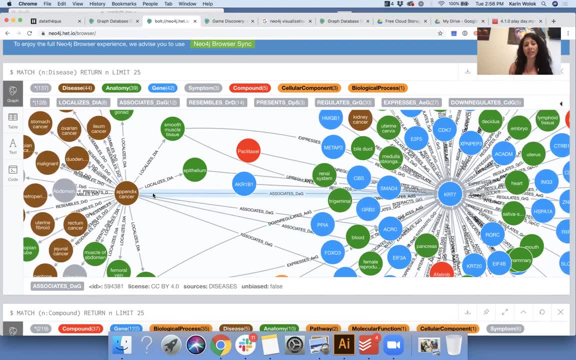 to support this type of data model, this highly connected data model. So when you're doing a query with most relational databases you're indexing and then you make another hop and you're indexing there and then you're another joints- all these joints are always indexing. 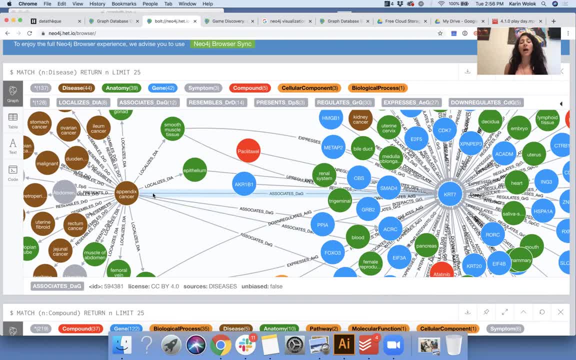 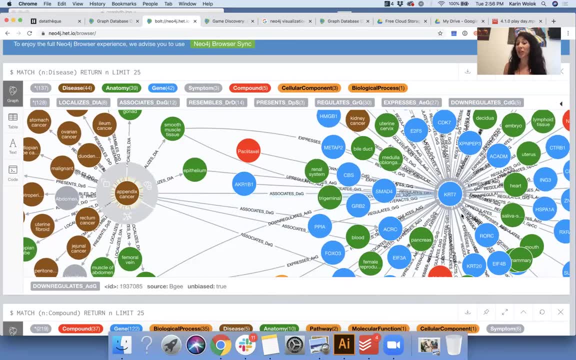 And that's very computationally expensive when you're doing a lot of hops With Neo4j. when you do a query, you index to find your initial starting point And then from there you're just basically chasing memory pointers, which the computer happens to be pretty good at. So the benefit of that. 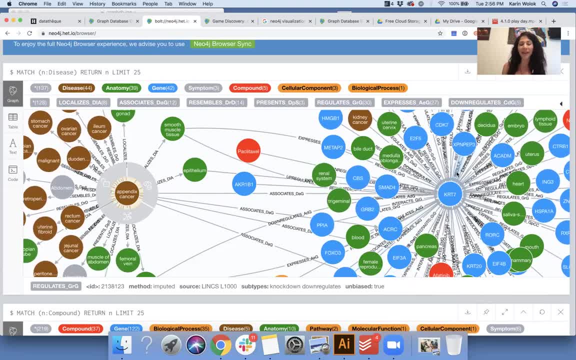 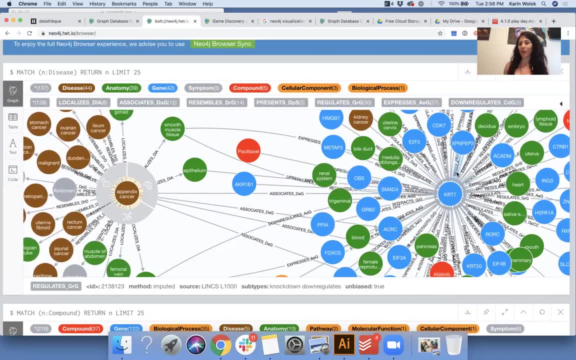 not having to index. you can index to find your initial starting point And then, from there, index every time you make a hop is pretty powerful. The traversal time between doing one hop or 12 hops can be pretty consistent, which is a pretty powerful thing when you're hopping. 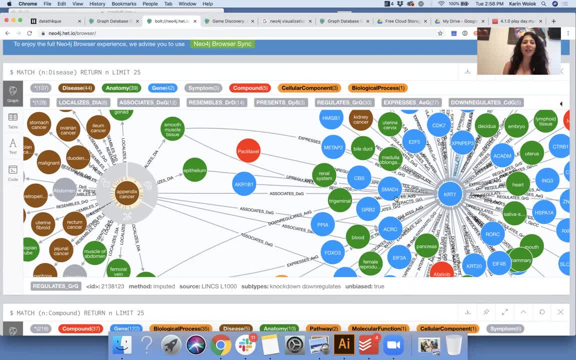 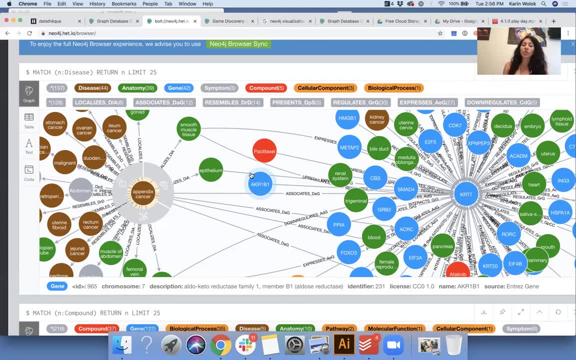 through a very, very highly connected network of things. So that's one thing that's very important to understand. And then the other thing is also the query language. So you're probably used to SQL because that's like a pretty standard query language. The problem is is that when you're 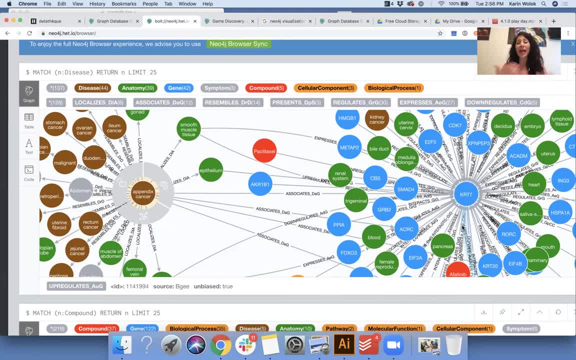 working with graph databases and graph type of problems. SQL isn't going to cut it because SQL is not built for highly connected data. So Neo4j actually developed language. It's an open language. A lot of other companies are using it. It's called Cypher And Cypher is a. it's basically SQL for. 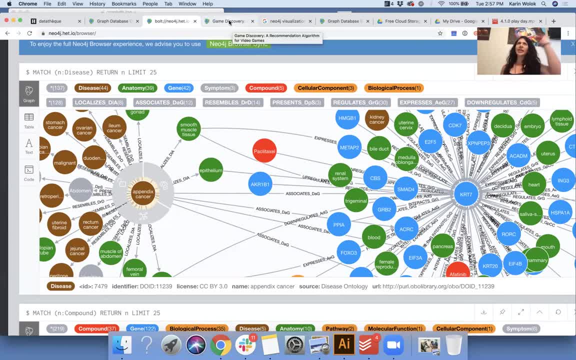 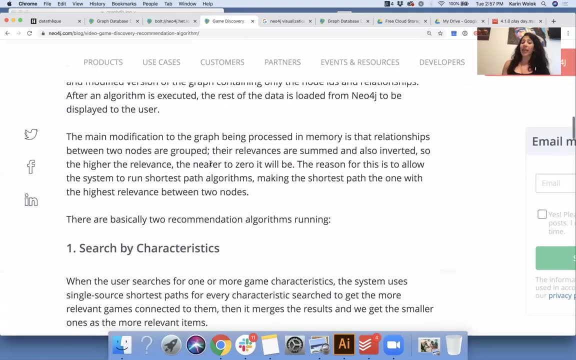 graphs. It's more like where SQL is kind of like: give me this like Cypher. you could be a little bit more ambiguous. It's based off of pattern matching, like more network-y kind of related, related queries, which is really powerful. So SQL is a declarative language And it's also 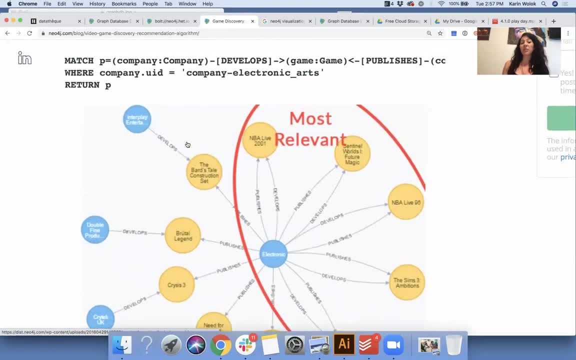 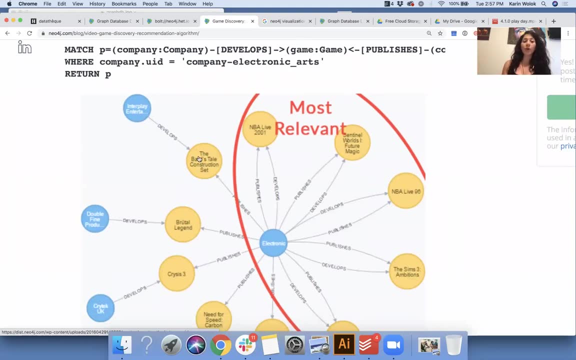 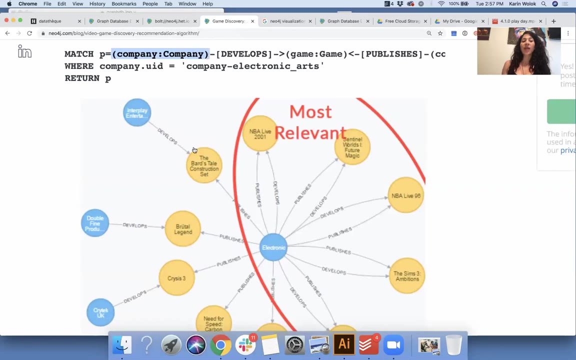 based off of ASCII art, which it makes it really nice to be able to see because it looks like what it actually represents. So just a high level overview of it. Your nodes here right In yellow blue: these here they're represented by parentheses, See. And then these relationships. 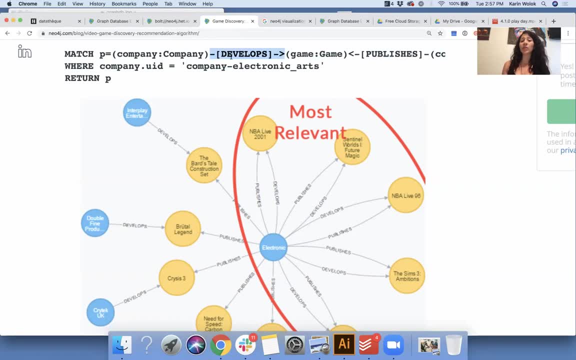 that are directional relationships between those nodes. R an arrow, literally an arrow, and then brackets with. it's almost funny to like. look at it, You're like, oh yeah, that makes sense. So here's another node, right, So it's. 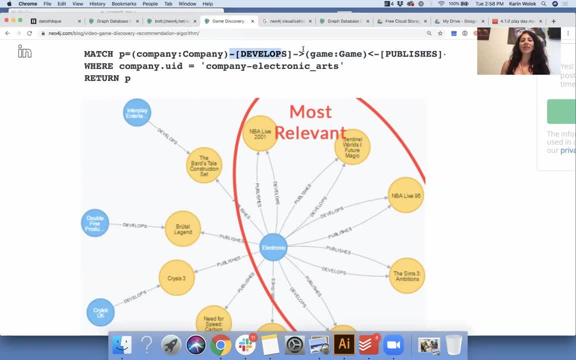 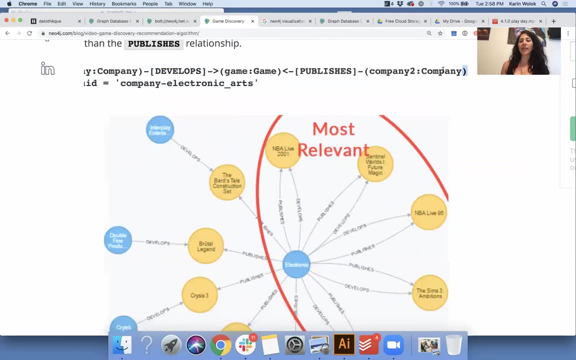 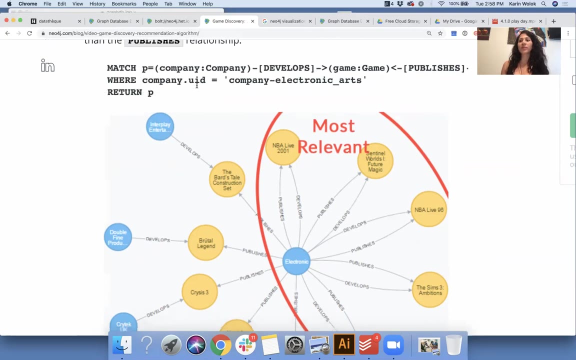 like we're looking for a company company that develops a game, But we're also looking for- there's another relationship here on this side- where a company also publishes the game, where the company is Electronic Arts. Wow, right, I know it's crazy. 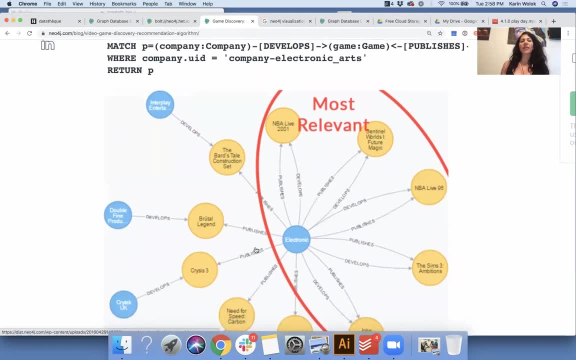 It's crazy. So I really like this blog post because I think it kind of shows the power of the model in general, like the data model, like being able to do a lot of these hops, But I think it also shows the power of having a query language that can help you. 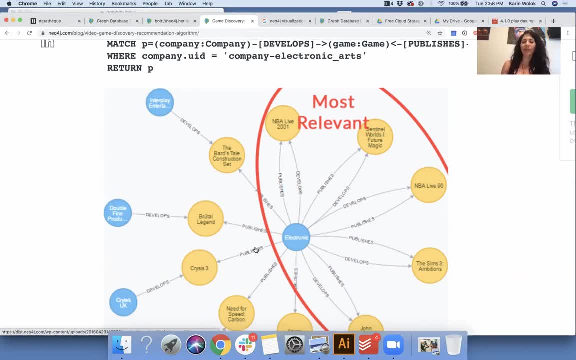 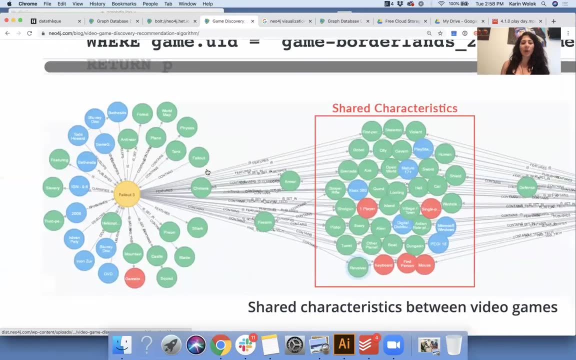 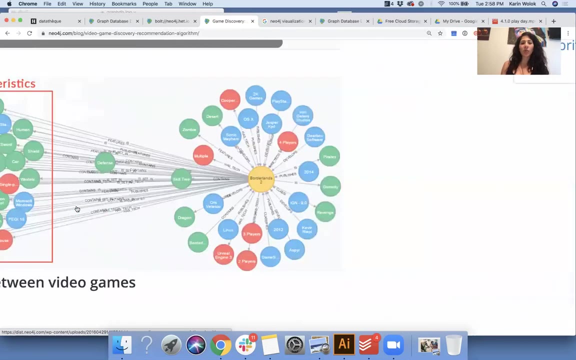 look into networks and graphs and patterns and pathways. It's just very cool. So I'll show you another example. This one, I also think, is pretty powerful. So here is an example of a video game recommendation. right, So you have a video game in the yellow node, that's fallout 3, and here, whoops too far. yeah, you have borderlands. 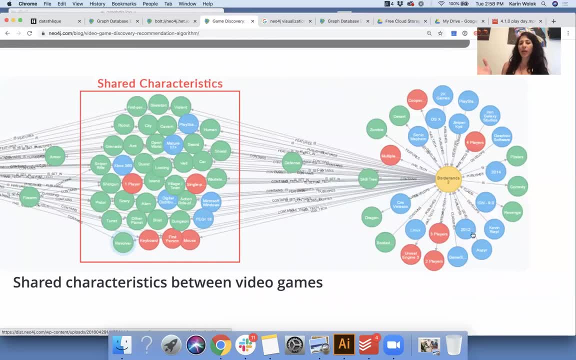 too right, and in the blue nodes they might be, i don't know, like consoles that the game is played on or whatever um. in the green you have different themes of the game. is it zombie and pirates and pain and war or whatever? um, and remember too, like these relationships because they're first class. 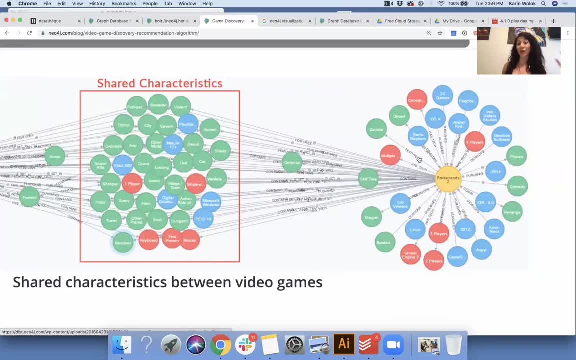 citizens. you could also have values on them, so they could be weighted. you could have a lot of pirates and a little bit of zombie or whatever, um, so that part is also something that you could take into account, which can be pretty powerful when you're, like you know, trying to make queries based. 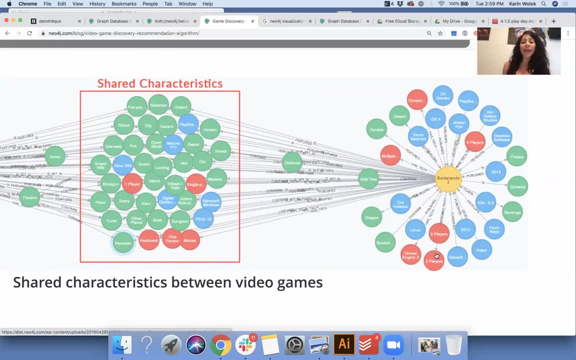 on weights, um, and then in red. you could have, like: how is the game played? is it played multiple player? are you playing one player as a first person, or with a mouse or a joystick or a keyboard? like how is the game actually played? now, here you, if you have a user that likes both of these games. 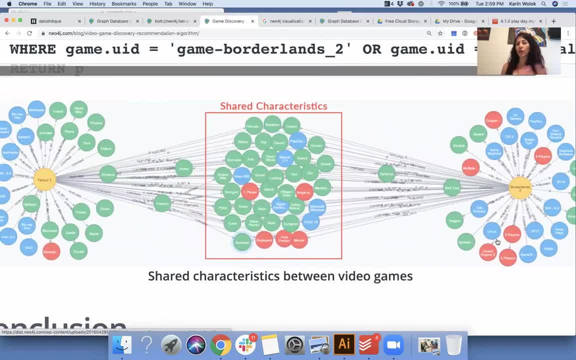 here and you want to say, okay, i want to understand who my user is, or maybe like find out what these two things have in common, so i could find another game that has the most in common with these two games. right, just generally characteristics like what are the characteristics of the game and what? 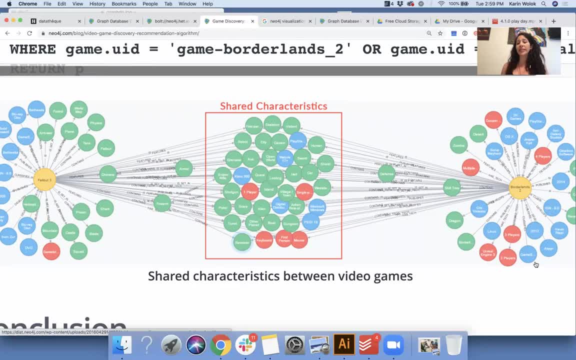 do they have in common? if you were to do this in sql, it would be a very extensive query because of all the different types of nodes that you have and the different types of relationships, um. so with cypher it's actually very, very straightforward. you might actually laugh at. 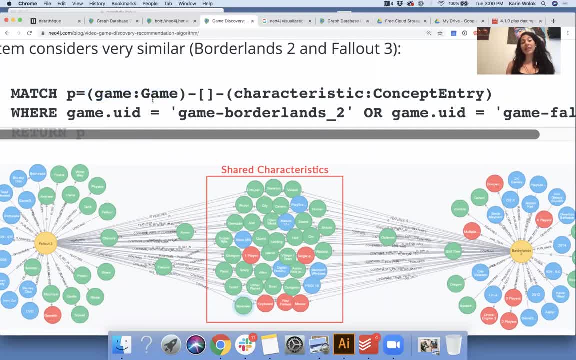 how amazing it is. but um, so this is an example of the cypher query. for this query, no, it's crazy, it's three lines. so you have here is like your node in parentheses. and then here is where your relationship would be, in this case the relationship. 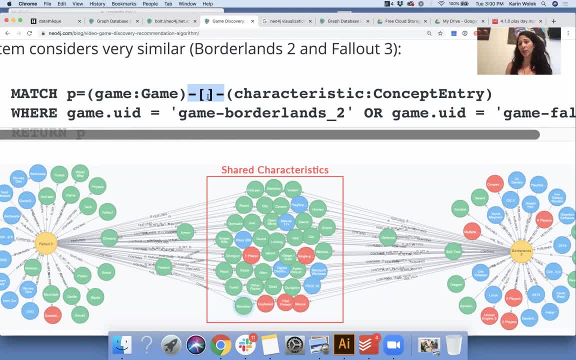 is undefined. any relationship, any direction. you could put a star six in there or something. if you want to look, six hops out or whatever. there's all kinds of different things you could decipher. um, but you're looking for, uh, characteristics and a game relationship between these two games. 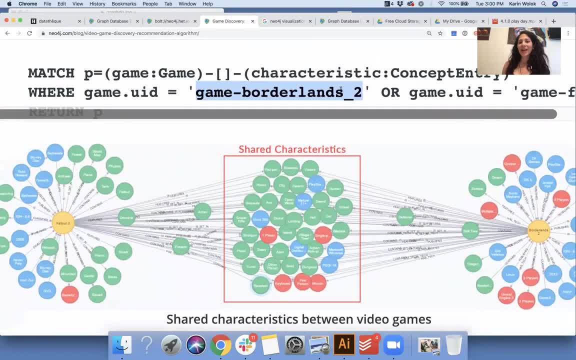 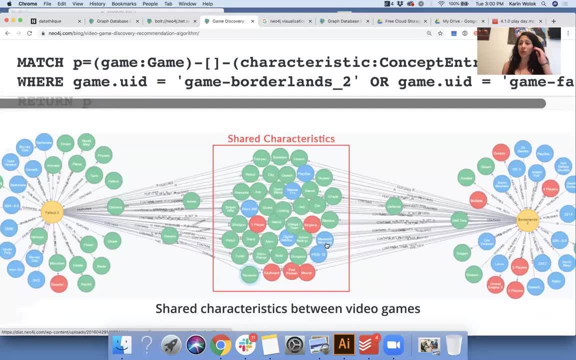 damn right. i know it's amazing, um. so this is, like i think, just like a really powerful example of like something you could do with not just the data model- like being able to store the data and query quickly, um- but also the ability to use cypher to kind of help you find the things that you know. 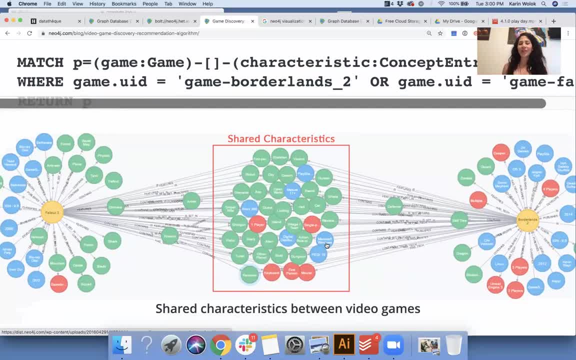 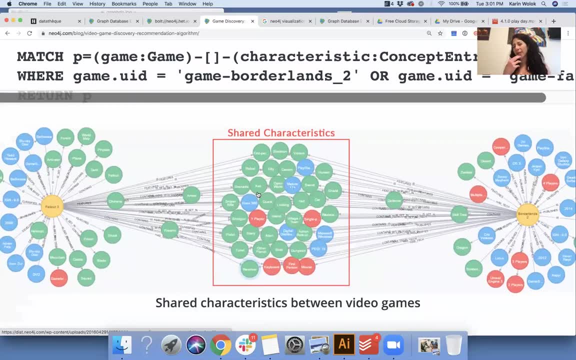 are normally highly connected or distantly connected or you know those like graphy related kind of problems. um, so i know you're probably already thinking about like, oh, where can i use this, because this does sound kind of interesting. um, i will tell you, there's a lot of really cool. 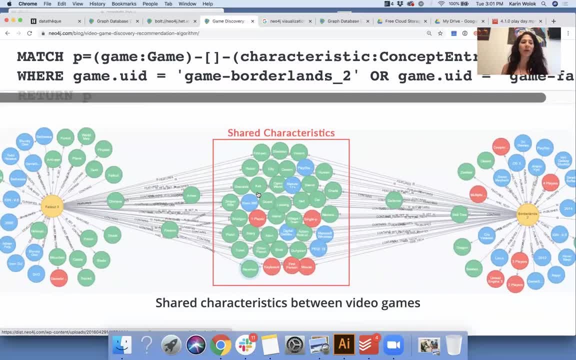 use cases for it, the very standard ones, like recommendations, um big one fraud detection, like network and it management. those are like the really big ones. that kind of uh are frequently used. um a lot of like nlp related stuff, like even if you think about linguistics. 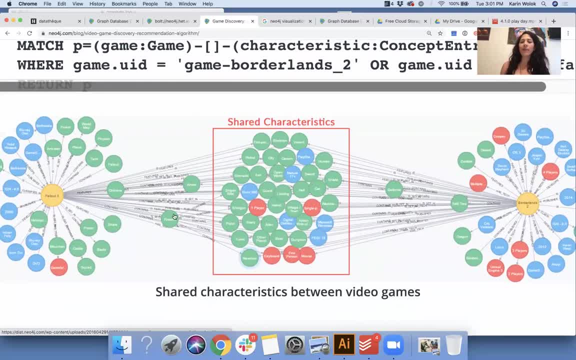 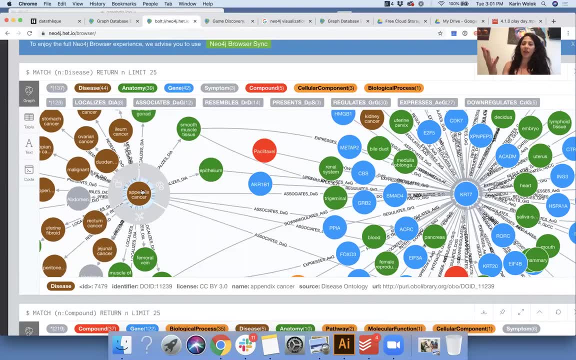 like how we speak, right, that is all a graph. um, there's this thing that happens that we call it the graph epiphany. uh, basically, when you start seeing in graphs everything, you see graphs everywhere- you can't get rid of it because everything's dependent on something else. you